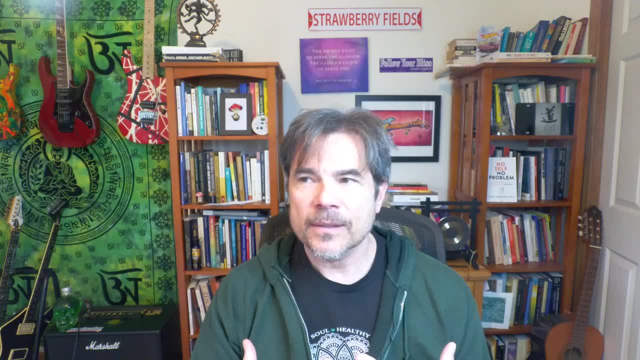 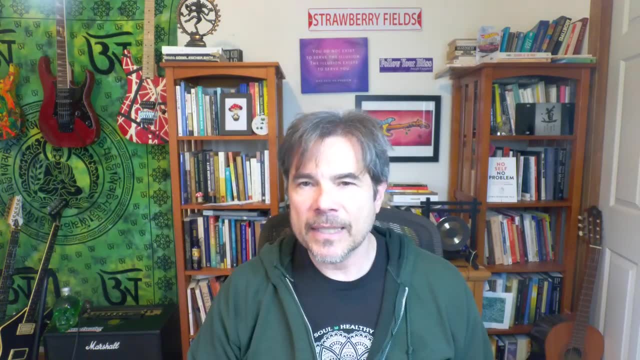 And by far the best has come from Rudi Rucker. So Rudi Rucker is a mathematician who wrote Infinity and the Mind, And when I came across his way of explaining it, it instantly became the way I talked about it in lecture. And not only did I talk about it in lecture, but I actually 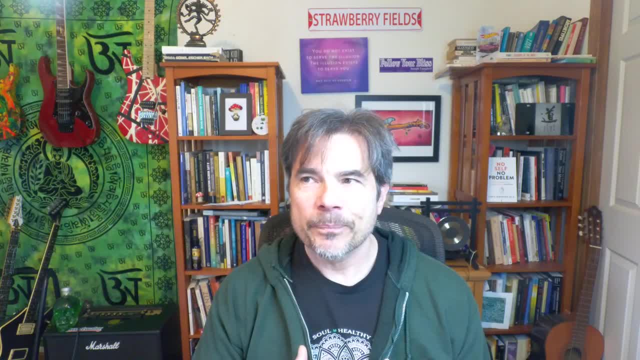 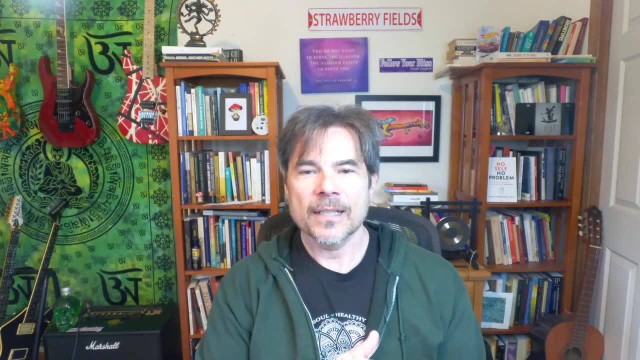 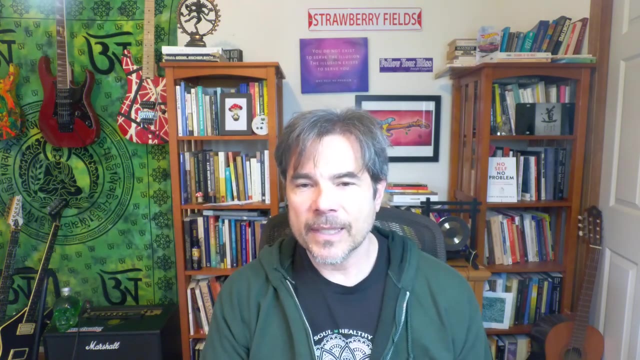 used his method as part of a scientific research project that ended up getting published, And I'll talk about that right after I discuss the theorem. So again, if you get Gödel's Incompleteness Theorem, if you get the original theorem, it's not going to make any sense to you. 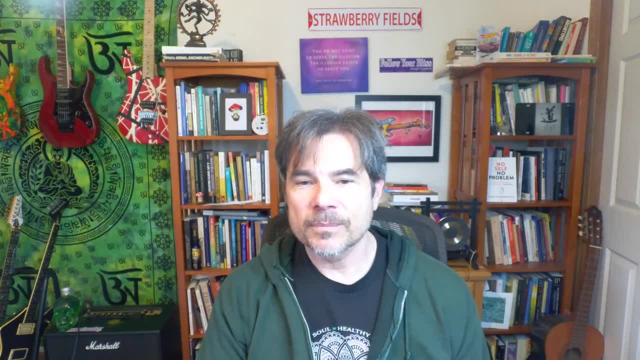 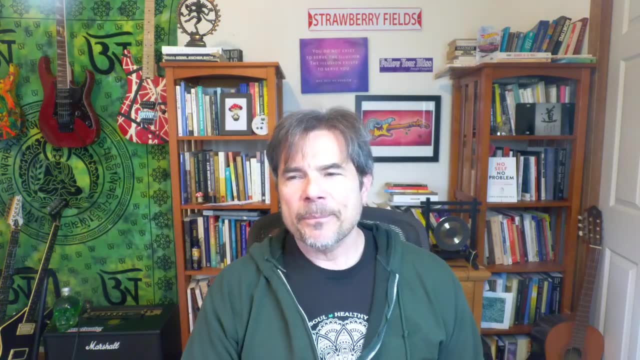 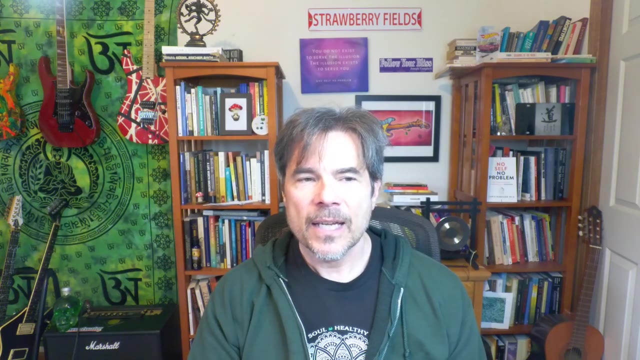 In fact, you pretty much have to have a PhD in logic just to even begin to understand some of the symbolic reasoning in it and these things called proofs. But the reason it's so important is because, even though most of us will never really get it in its entirety, you can get a. 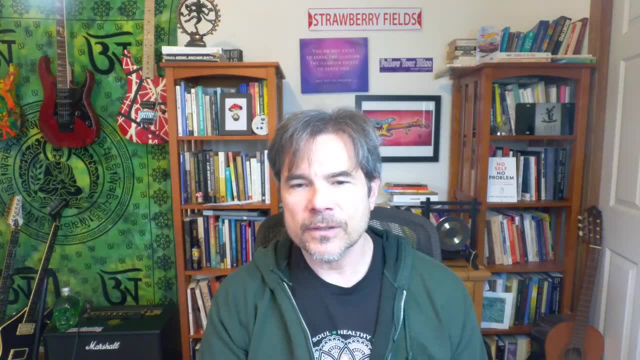 version of it, And that's why I'm talking about Gödel's Incompleteness Theorem And I'm not going to give you a version of Gödel's Incompleteness Theorem in this video, A version of Gödel's. 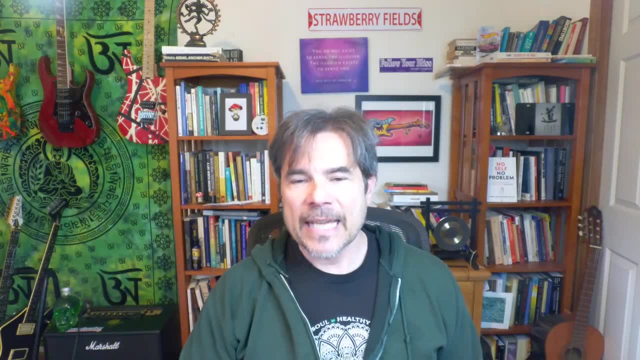 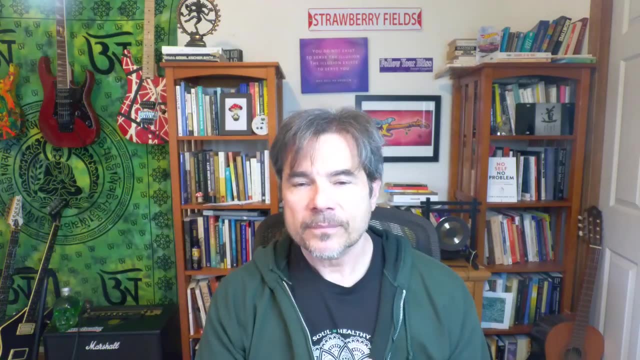 Incompleteness Theorem that us ordinary people can get, And when we get it, we get the importance of it, And I'll talk about that too when I'm done. So let's get into it. Okay, so this is again based on Rudi Rucker from Infinity and the Mind, And he says: 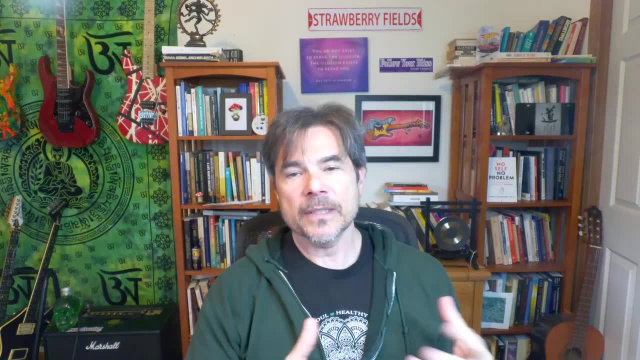 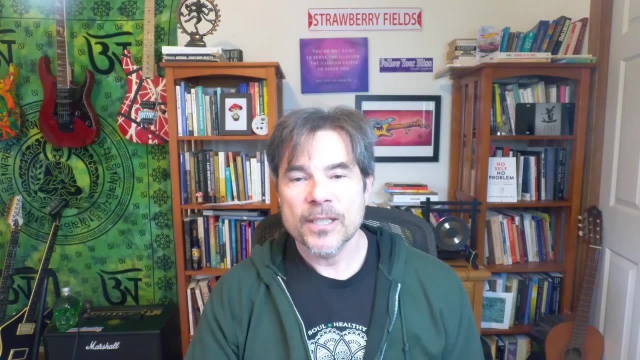 let's imagine there's a universal truth machine. This is the most sophisticated, advanced computer imaginable, And let's just call it UTM for Universal Truth Machine. It can state any truth in the universe, And that's because it's so ultimately intelligent and advanced, And so 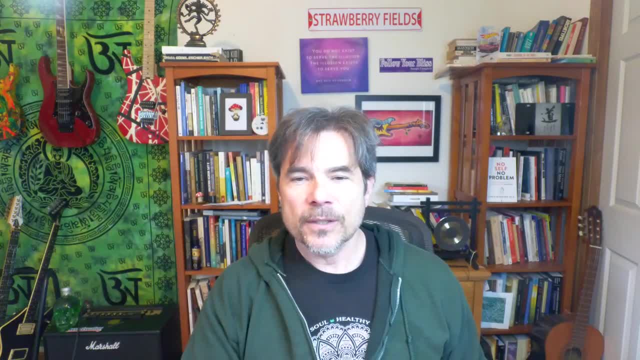 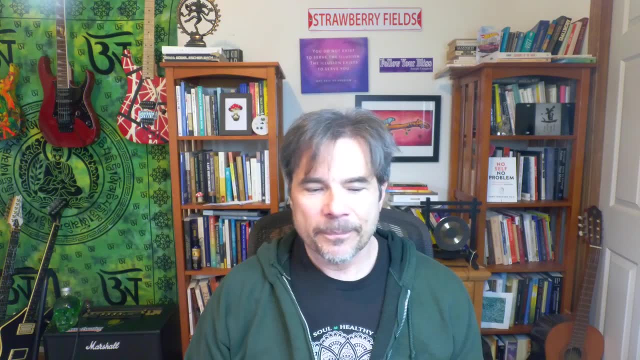 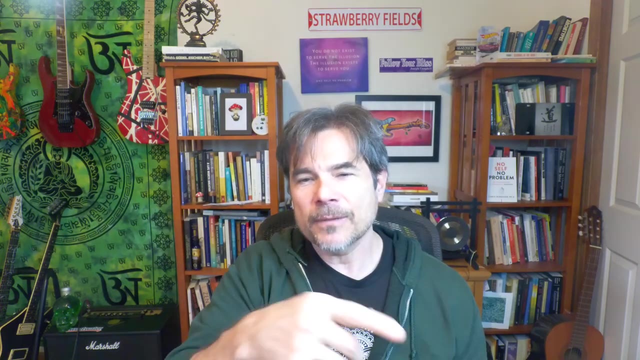 here we've got UTM, the Universal Truth Machine. Now Kirk Gödel is very clever, So what he wants to do is he's going to back this machine into a corner, And I'll show you how he does this. He writes out a sentence: UTM will never say. G is true, But here's the self referencing part. 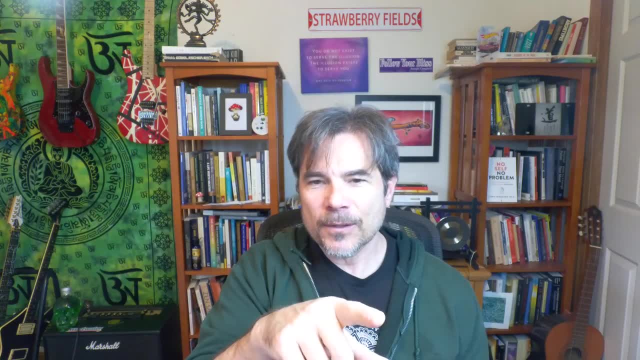 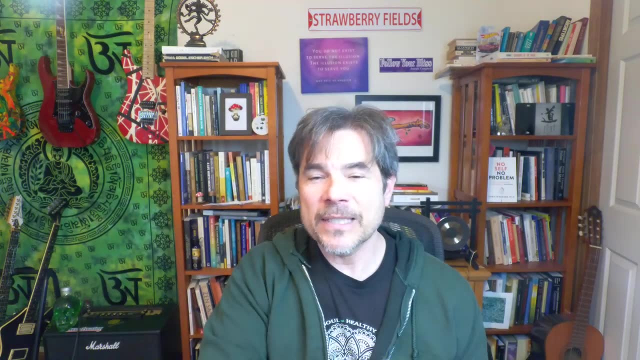 but let's go slow with this. He actually creates a reference to this statement. So the statement itself is: UTM will never say G is true. Then he calls that statement G. So here in all my technical sophistication, I'll let you kind of ponder that for a little bit. 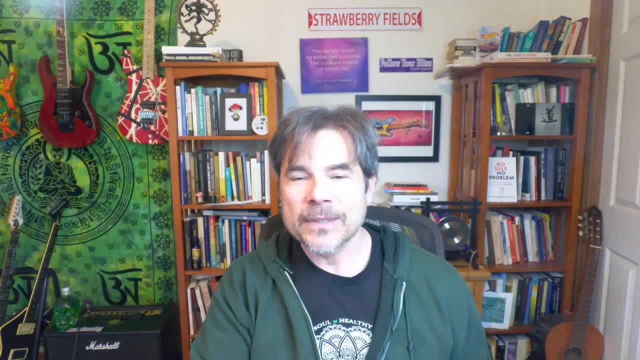 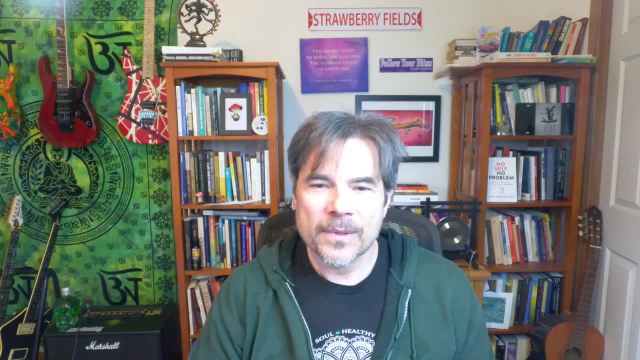 So G is the statement. UTM will never say G is true. Now he writes this out, just like I did to you, And then he shows UTM the statement and asks: UTM, is G true or not? Now here's the cool part. if it hasn't hit you, you better see it. This whole system doesn't allow you to complete the command statements assembly just because of some nice little prophecy, like he didn't do, And that would involve three parentheses. but when I worked at the time of the велicodium meter, I showed you. 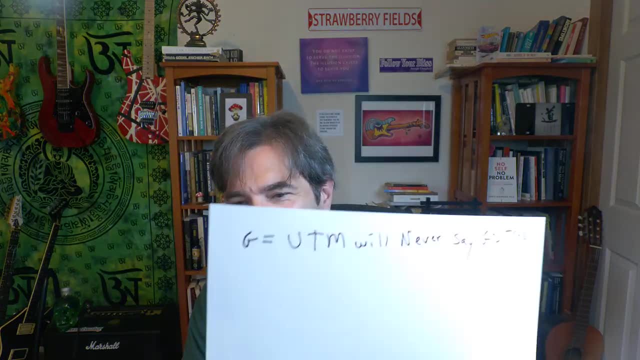 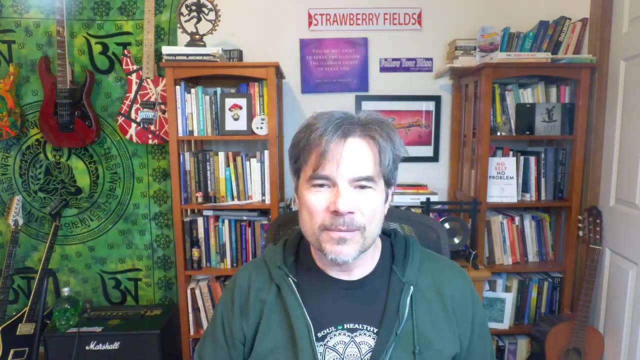 the weather instrument element that is. I don't know what the word does, so fingers crossed. I was trying to keep everything all you need, but it was hard to do. And here's thegebenation hertz too it So again, by staring at this, imagine giving this to UTM. You backed UTM into the most. 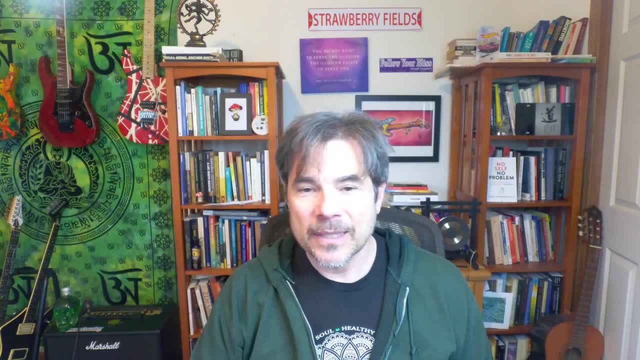 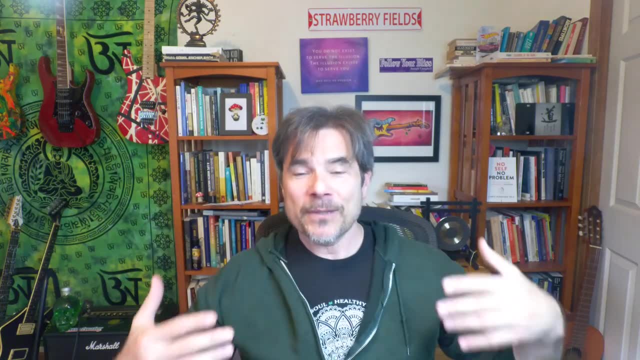 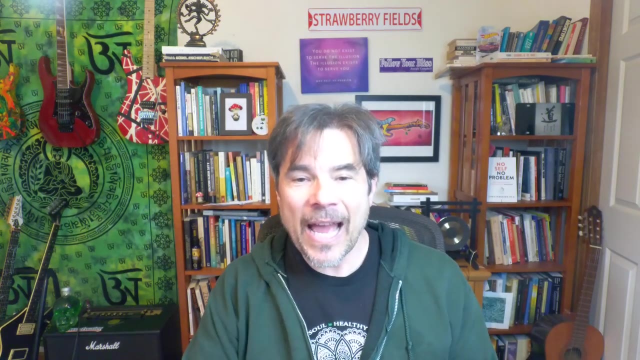 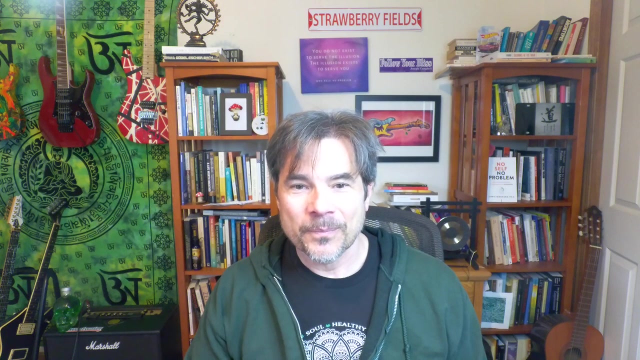 metaphysical, cosmic corner possible. If UTM says G is true, it makes it false. So UTM, this machine, is supposed to be capable of stating any truth possible. It cannot say what is actually true and in doing so, makes it actually true. Okay, and you may have to pause and go back a little. 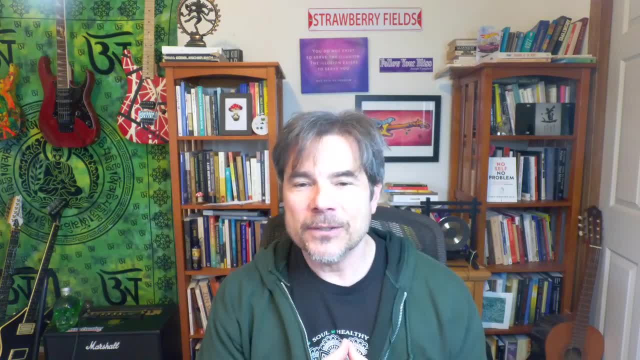 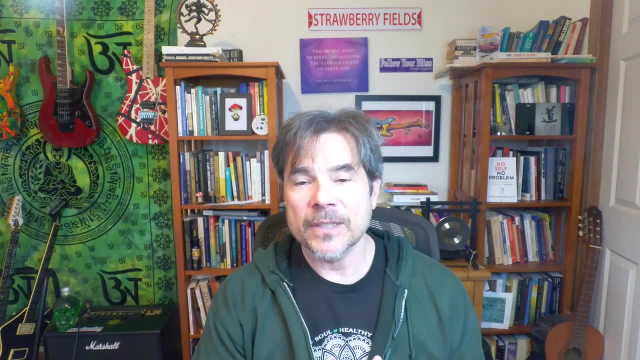 bit and do that a few times. What I found in research- and I gave this to a couple hundred students- what I found is that for some of them it absolutely clicked very quickly And they found the paradox in it. And these were mixed handers, people who have a larger 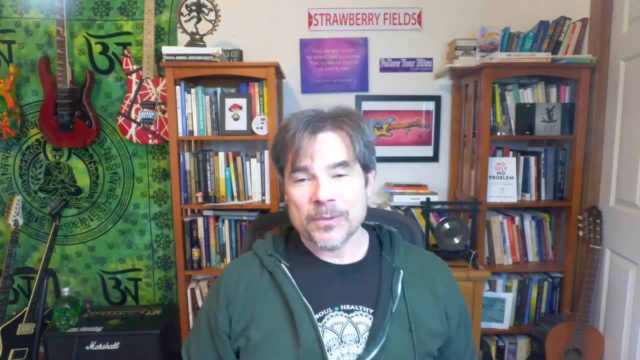 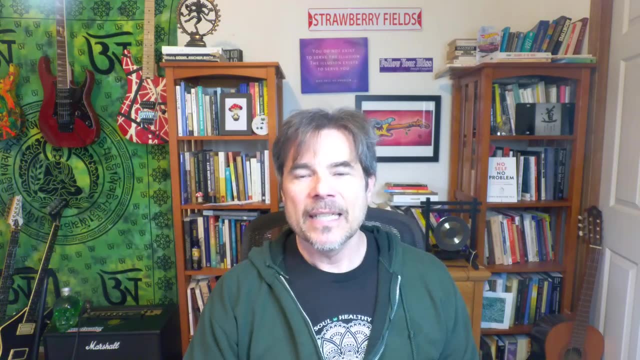 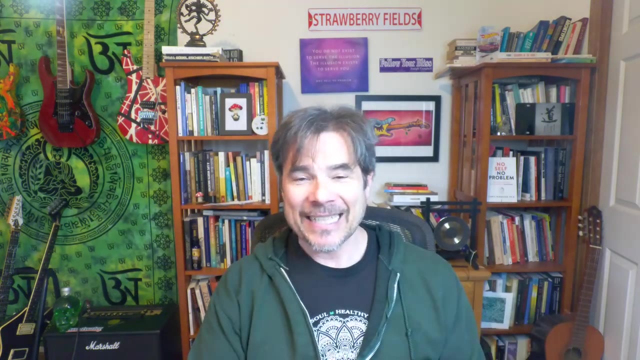 connection between the two sides of the brain. For other people it was really difficult for them to make, for them to feel it And, honestly, when I explain it in class, I don't get the same sensation, because it's very difficult to focus your attention on explaining it and getting it. 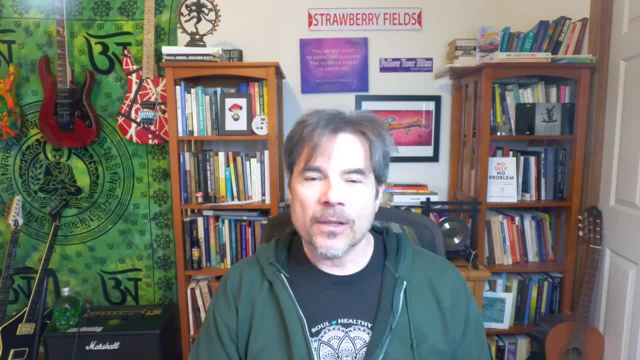 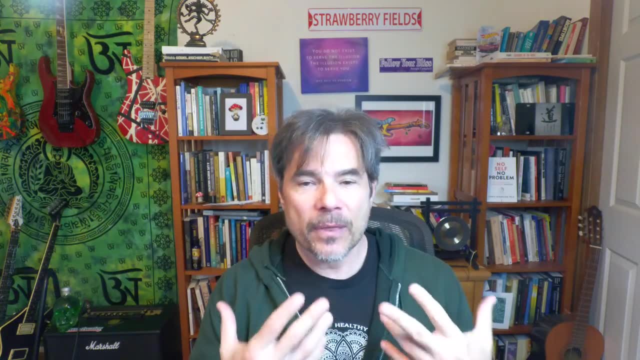 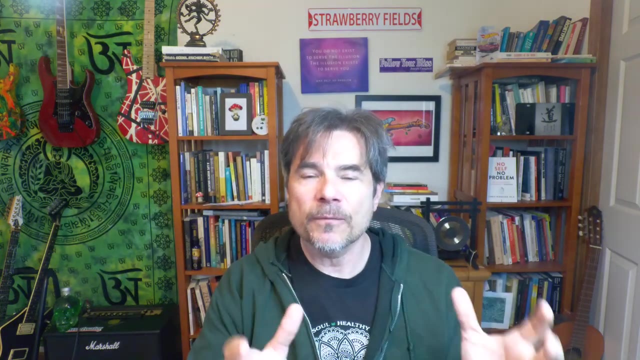 at the same time. But the wonderful part about all this is what it implies as far as consciousness and mind is concerned, and particularly, at least in my view, the thinking mind. What he was able to show is that the very best, most intense form of thinking. 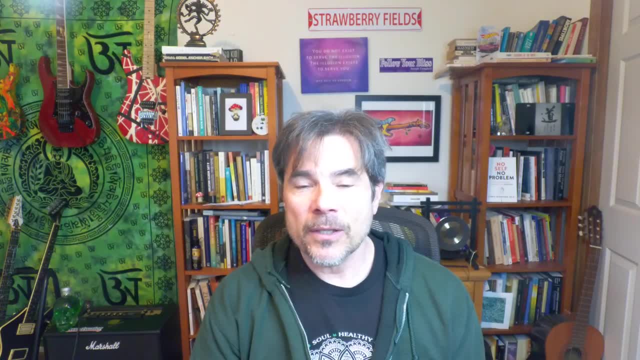 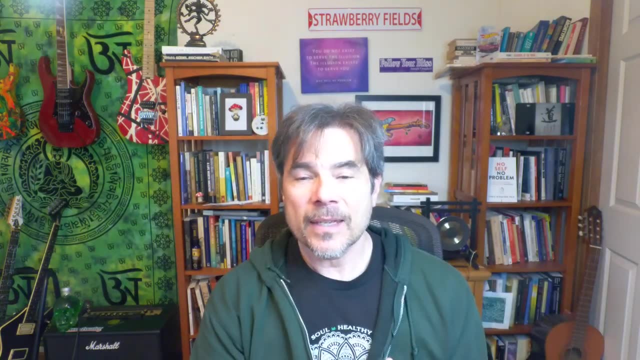 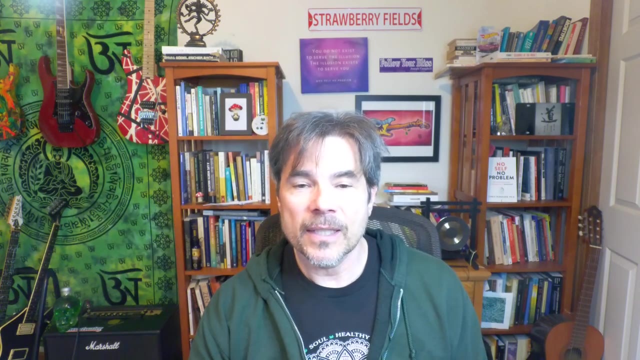 results in a really clever paradox where, if you put thinking to the test, it will ultimately come up with absolute proof that the thinking mind is limited and that there are truths, things that are true, that are way beyond the capacity of the thinking.